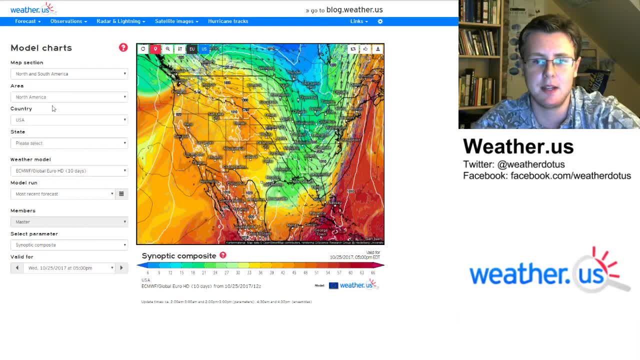 to synoptic composites. That's what we're going to be looking at today, And you're going to get a map that looks kind of like this. So what does this map show? It shows a bunch of different things. So the shading in the background here, these reds fading down to the blues over here. 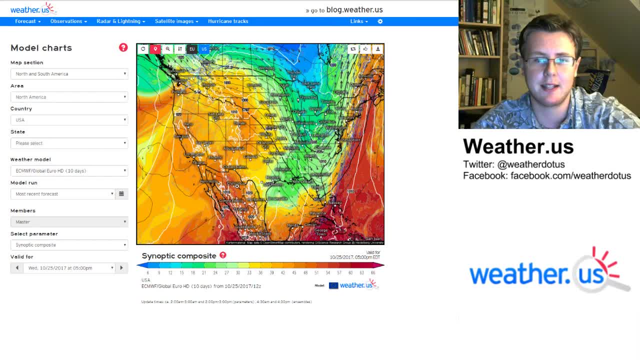 this is a parameter known as theta E. While that sounds fancy, it's basically a measure of heat and moisture in the atmosphere. So higher theta E values indicate warm, humid air, whereas low theta E values indicate cooler and drier air. So that's basically a. 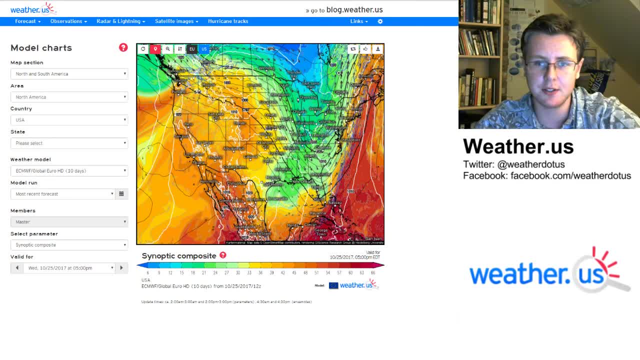 little bit about theta E. The vectors here are upper level wind vectors, so the jet stream level. So that shows you basically where the jet stream is, how fast it's blowing and in what direction it's blowing. So those are the vectors, The black lines here. 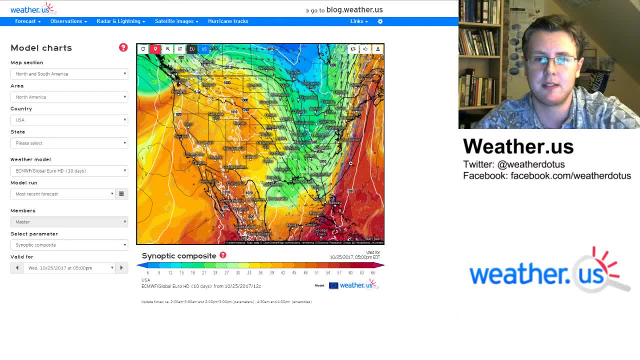 are 500 millibar height contours. So it's the level. how high up would you have to go in the atmosphere for the pressure to be 500 millibars? And then the white lines are sea level pressure. so that's just atmospheric pressure at the surface. So what does this composite do for us? 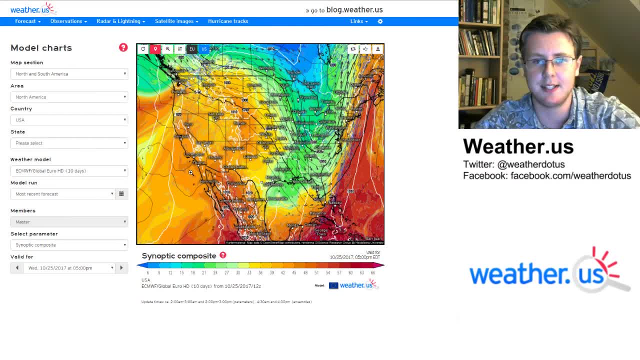 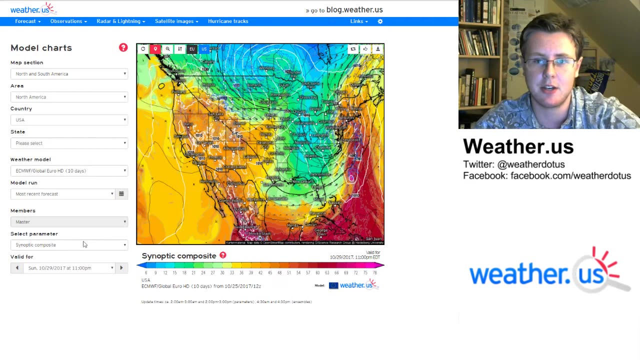 Well, it allows us to see a number of different large scale processes that can bring some fascinating weather. So, as I'm making this video, we have a very big storm forecast, potentially in a few days from now. So I'm going to just click to that because that'll kind of show you. 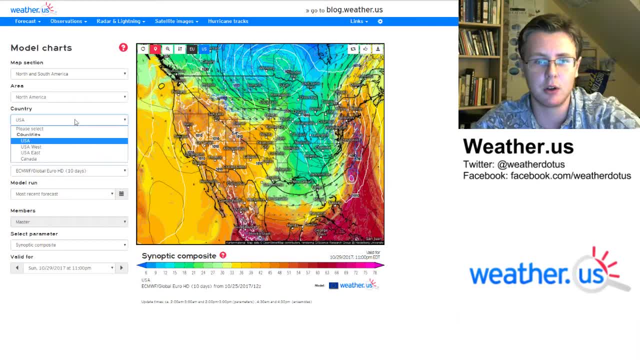 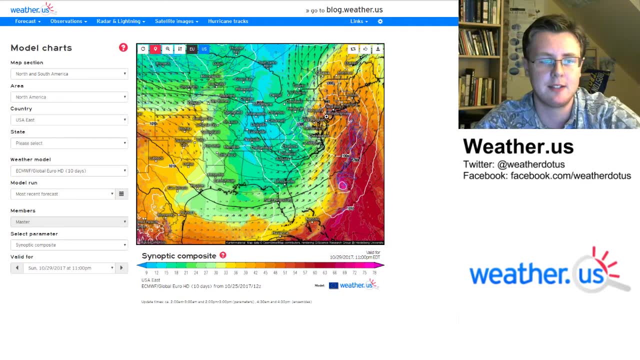 give you a sense of what this parameter looks like in a real world storm situation. So I'm going to zoom into the east coast, because that's where this storm is forecast to be centered. So here we are. This is basically for what's going to be close to the height of the storm. 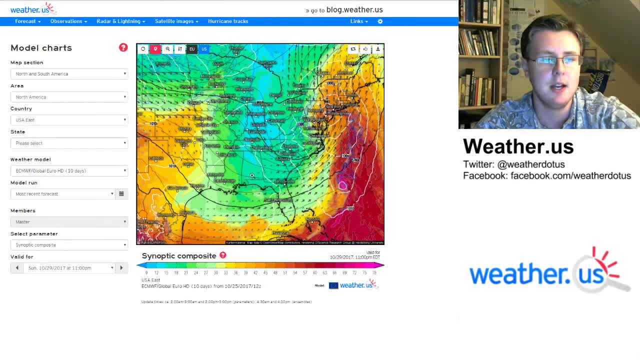 This is forecast a few days out from what I make in this video. You can see on the MSF data that this is probably the highest level that we have so far. OK, this is a very deep trough. it's at an altitude of about 164 feet. There's not a lot of ground in this trough. 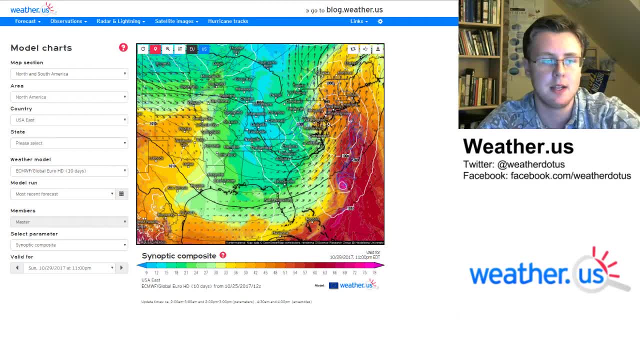 probably the mid-maxparameter worth. And then here we have a very low pressure center Just west of New York City. it's a very strong low pressure center, down below 980 millibars. That's quite strong, especially for this time of year. We have a deep trough at the 500 millimeter level. 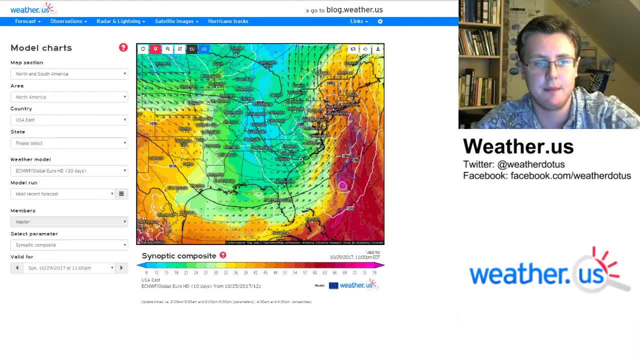 So you can see these contours dip down, And so you can see that the axis of this trough is oriented with a negative slope, so from northwest to southeast, And you can see that it's looking like this at the bottom of the map And, as you can see, the surface is more or less. 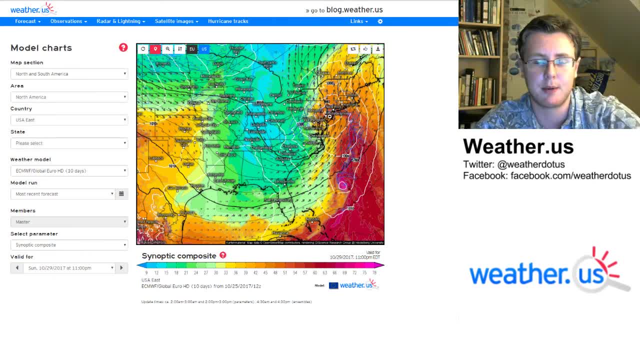 located behind the surface low pressure center. so whenever you have this backward tilting system as you head from the surface to the upper levels, that indicates that the system is going to continue to strengthen until that upper level disturbance catches up to the surface storm. so this map is showing us that we have a low to mid-level environment very favorable for 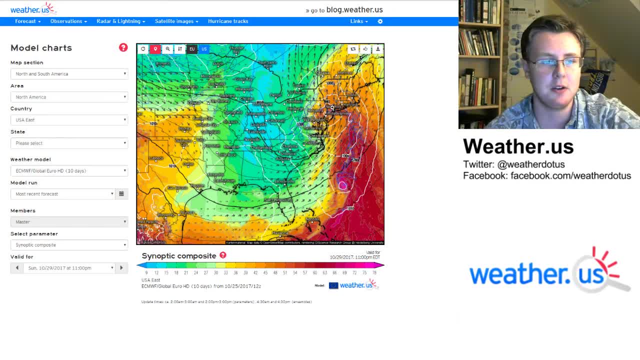 continued storm development. another thing to note is that this storm is located within area, or near an area of very high theta e values. so there's this little tropical disturbance. you can see a theta e maximum near there, but this axis of very high theta e values indicates rich tropical 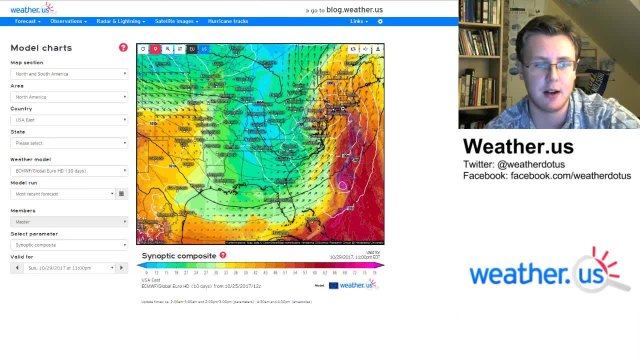 moisture is being brought up from the caribbean all the way up into new england, so this storm is going to have a heavy rain threat as well. the upper level jet stream vector is going to be 直接 switched to media indie. 짧아ary any. 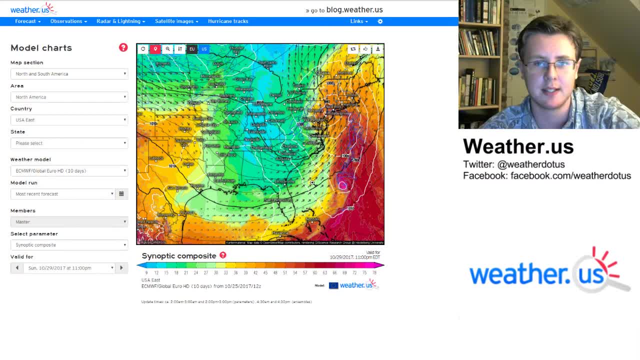 of you may have heard of theúlt вещиpoor, 시바걸아 ויע Elli the taking this out of the southwest, and then you have another area of strong winds that kind of bends around s, around you know where. 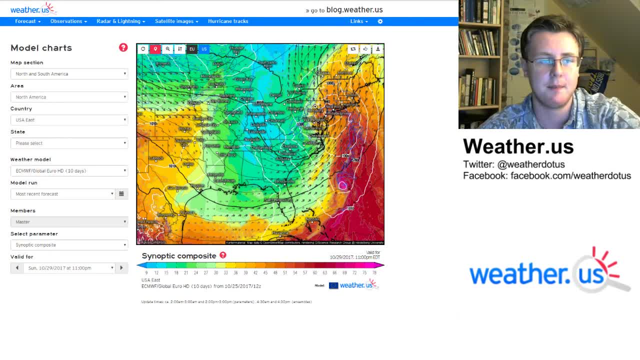 the storm would probably be removed. the southeast and then out of the south, basically extending from central Pennsylvania, western New York up into the portion of eastern Canada, here, Ontario, between Ottawa and Toronto. So you have these two jet streaks. air likes to rise kind of on the left side of the exit. 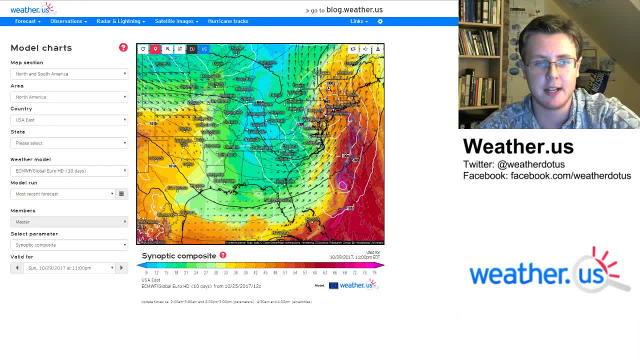 region of the jet streak and it also likes to rise on the right side of the entrance region. So when you have these two areas kind of co-located, which they are in this situation, then that's an additional factor to support low-pressure development. 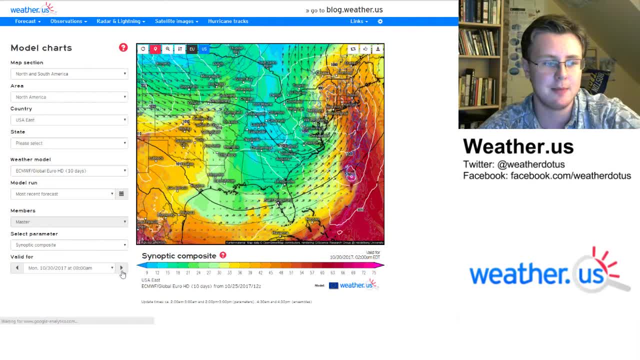 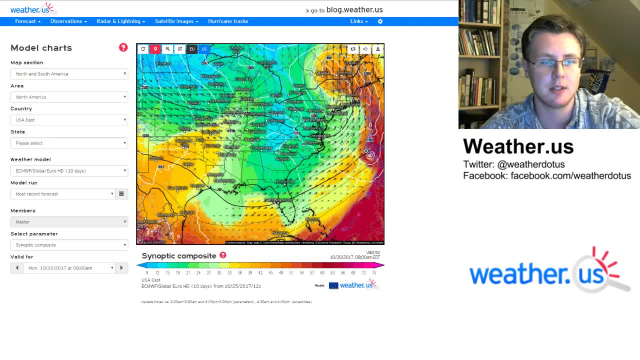 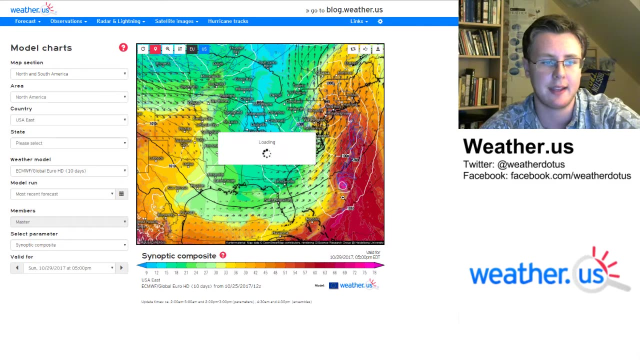 So basically big storm. it remains to be seen a little bit how much this energy can phase into the storm or not. So this run kind of keeps that tropical system off to the south and east. Some of the earlier runs had that getting kind of caught up in the circulation as a. 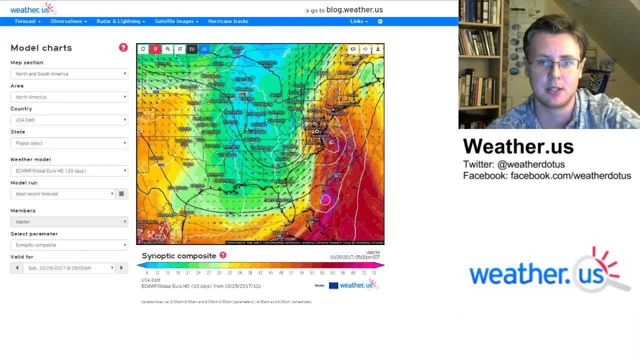 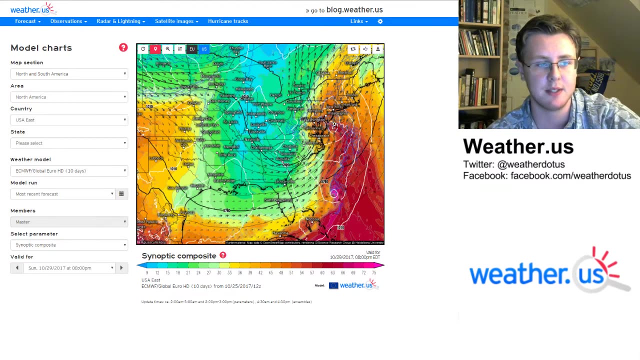 whole. But that's basically how you use this synoptic composite. You're looking for For high theta-e values. that indicates moisture, High theta-e gradients, sharp theta-e gradients. so when you have very high theta-e values located in close proximity to very low theta-e values, that's an indication that you have. 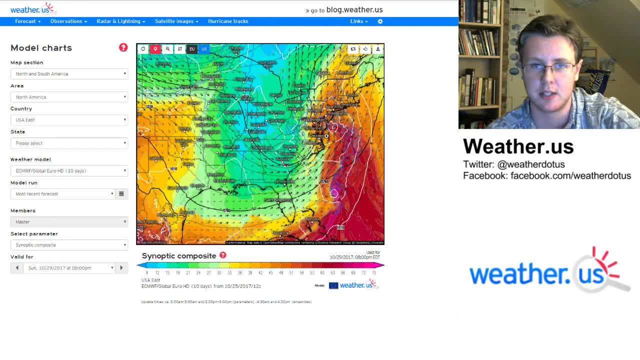 a lot of baroclinic energy, so that's basically energy that storms can use to fuel themselves. So again, that's another checkbox that we're ticking here. It's obviously not as strong as some of the big deep winter cyclones that we have. 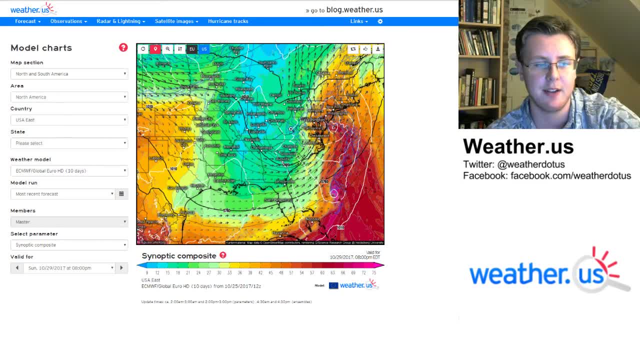 But you have this very sharp gradient. It's a gradient between high theta-e values and low theta-e values. One other contour that's plotted on here that isn't super visible is relative humidity in the mid-levels. Those are those little blue contours here. 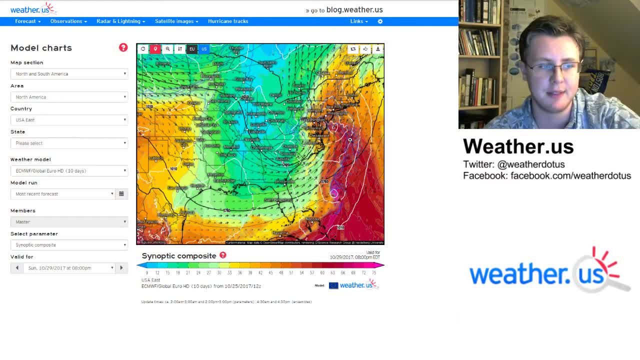 So that just indicates moisture. but you already have theta-e to kind of figure out where that moisture is. So these contours will give you a rough sense of where you might expect to find cloud cover. So that's relative humidity values 80, 85%. 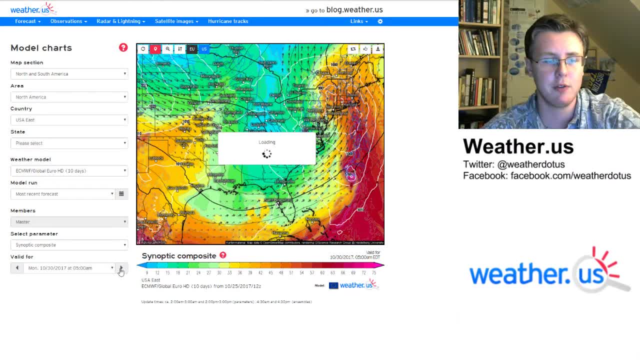 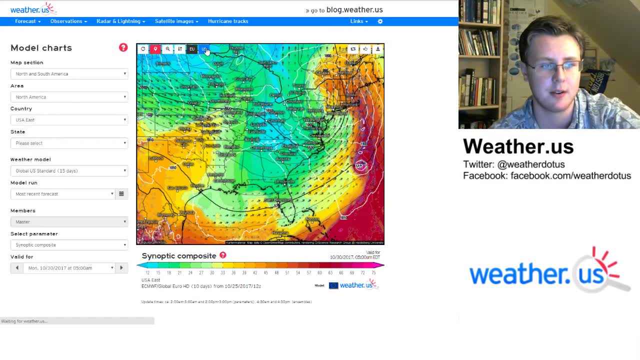 So that's basically a quick overview of how you use the synoptic composite. It's available for the ECMWF model and also the GFS model, So you can kind of use these to compare. in this situation ECMWF is a little slower and a little stronger with that storm. 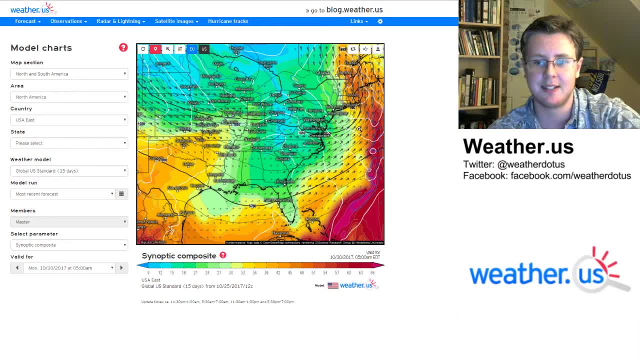 So we'll see how that plays out, but this should give you a good sense of how to use that composite. I hope you enjoyed the video and enjoy using this composite. If you have any questions, be sure to let me know. Thanks for watching. 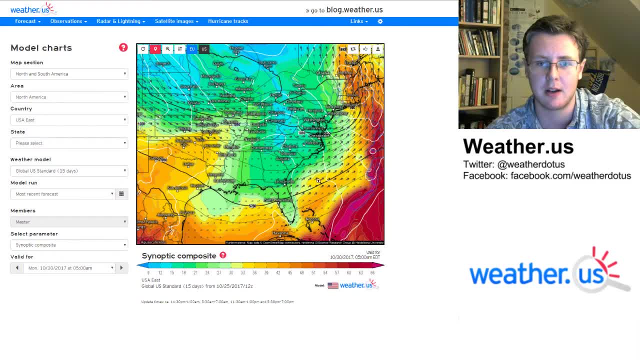 If you have any questions, be sure to let me know through Twitter, Facebook or comment on the blog. Thanks for watching.